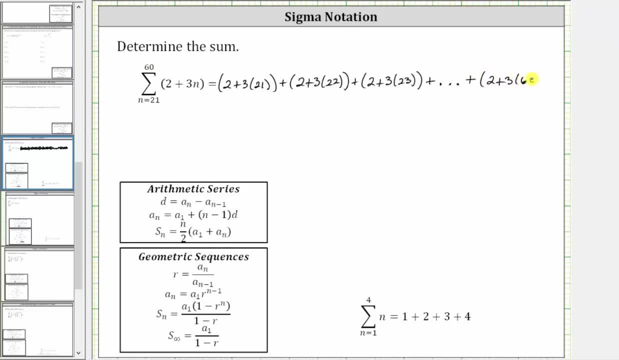 and therefore the last term is two plus three times 60.. And now let's simplify: Three times 21 is 63.. Two plus 63 is 65.. Plus next, we have three times 22,, which is 66.. Two plus 66 is 68.. 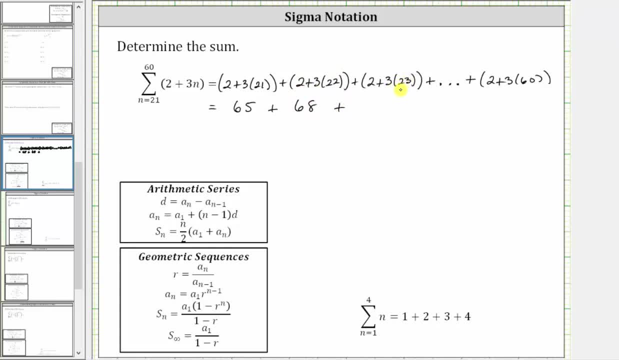 Plus. next, we have three times 23,, which is 69.. Two plus 69 is 71.. Plus. and then, the last term, we have three times 60,, which is 180.. Two plus 180 is 60.. 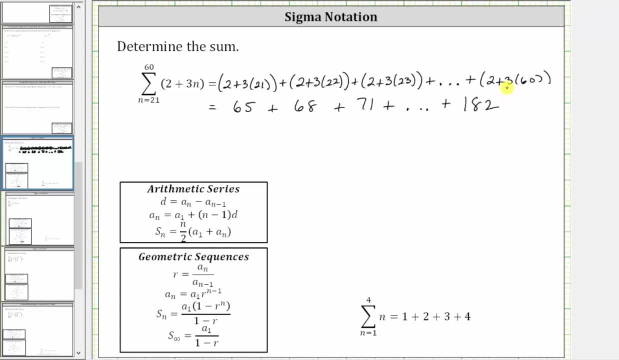 80 is 182.. So if we didn't recognize it before, we should now recognize we do have an arithmetic series, because the terms are increasing by three. So let's make a note over here. The first term, a sub one, is 65. 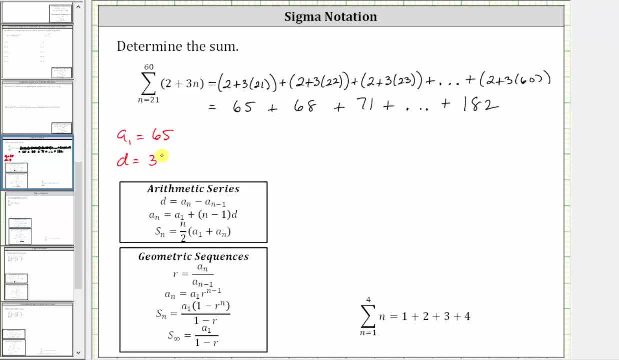 and the common difference d is positive three. Remember: if we needed to, we could determine the common difference d by using the formula: d equals a sub n minus a sub n minus one, which means we can find d by selecting any term in the series. 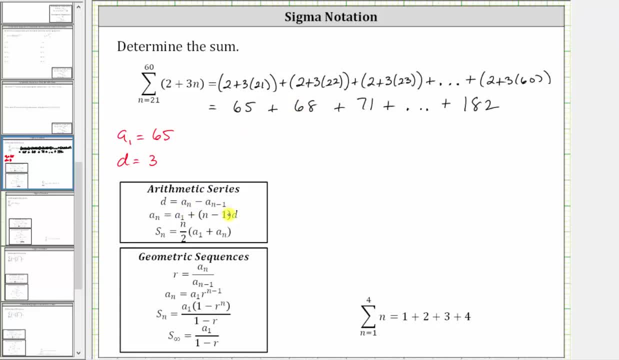 except the first term and subtracting the term before it. Notice, 68 minus 65 is three, 71 minus 68 is also three, And we know the last term in the series is 182, and therefore a sub n is equal to 182.. 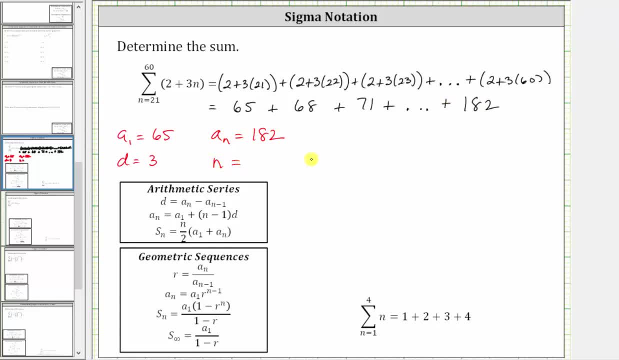 Now we need to determine n, the number of terms in the series. Well, notice how the index goes from 21 to 60. So we might be thinking we should take the upper limit of 60 and subtract the lower limit of 21. 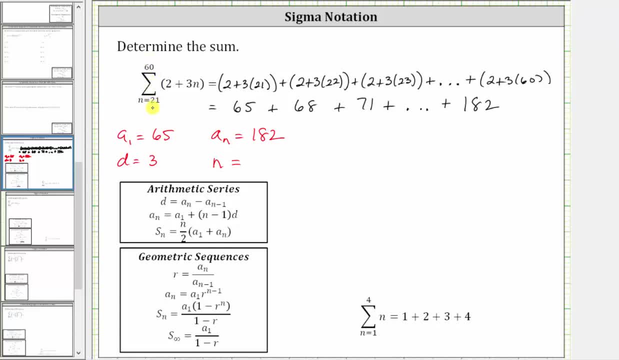 to determine the number of terms. But 60 minus 21 is 39, which is not the number of terms. There's actually one more term, or 40 terms. To better understand this, let's look at a simpler example. Let's say we have the sum from n equals one to four of n. 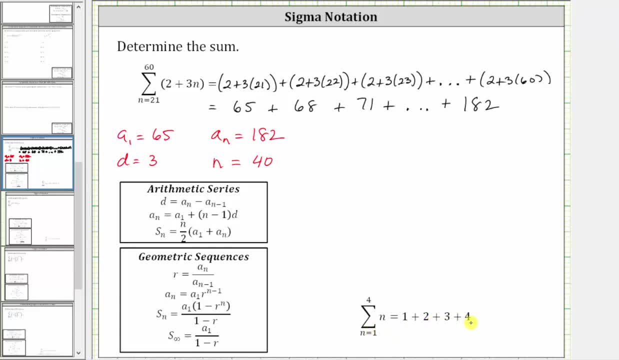 If we expand this, we have one plus two plus three plus four. We can easily see we have four terms. but if we take the upper limit and subtract the lower limit, we have four minus one, which is three, But again we have four terms.